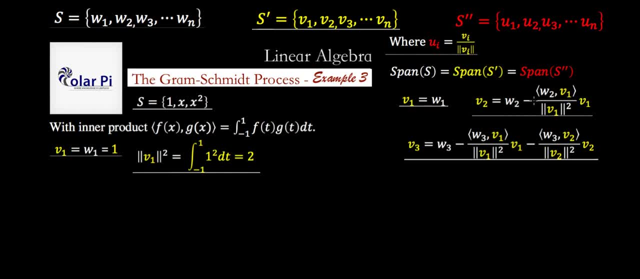 is X, right, Okay, But we need to figure out what this is right here, the inner product between W2 and V1.. And of course, for that we're going to use this inner product that we've defined. But let's summarize everything. 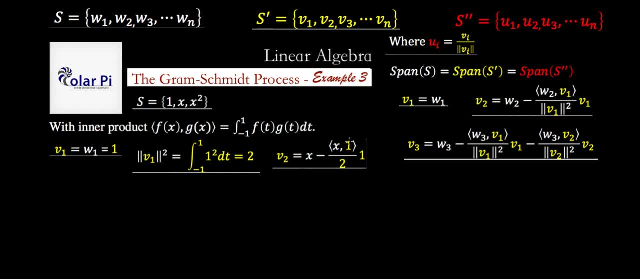 we know so far in writing this: Yeah, Okay, cool. And so again, the only thing left that we need to figure out before we say what V2 is, is this here? which again, is W2? V1 inner product? Yeah, this here. 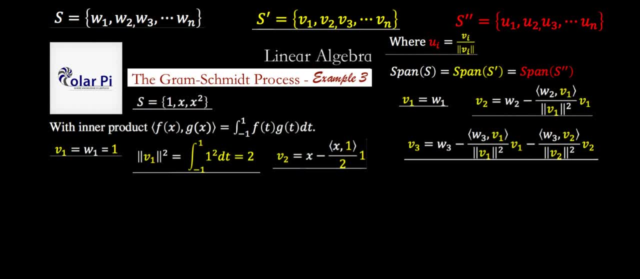 So, using the way we defined our inner product, we see that the inner product between W2 and V1, this here would have to be this here- which in turn is equal to zero, because basically, the integral from negative A to A, the integral from negative A to A of any odd function is zero. That's the 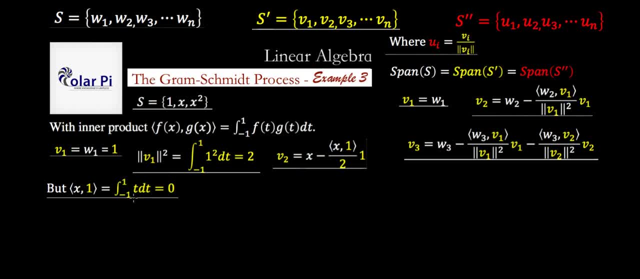 easiest way I can say why this is equal to zero. But you could also do it. You could actually compute the integral like carefully and see that it's equal to zero. So we're going to do that. But yeah, it's better that we say that the integral from negative A to A of any odd function. 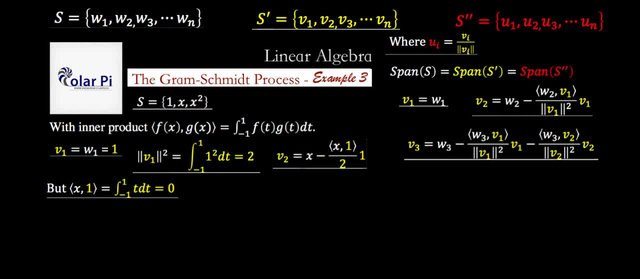 is zero, because we're going to need that fact again a little bit later. All right, let's move on. So, now that we've got this handy, it means that we know what V2 is completely, And this is V2.. That is V2 is X. Yeah, Okay, cool, All right. So far matching, All right, And so let's see. 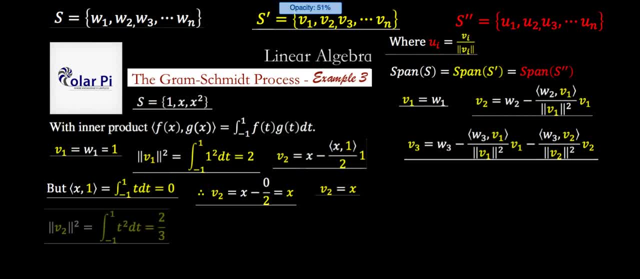 what is V3 going to be? Well, in order for us to figure out what V3 is, notice that we need to know what the norm of V2 squared is, And we also need to know what the inner product between W3 and V2 is, And we need 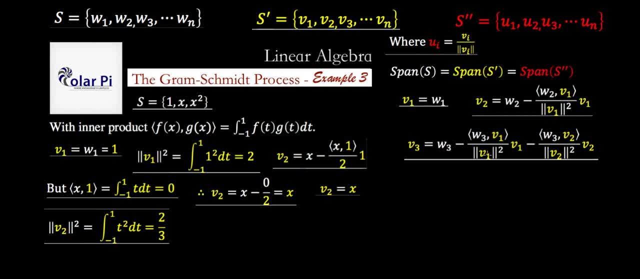 to know the inner product between W3 and V1.. We already had the norm of V1 squared from earlier. It was two. We clearly know W3 is X squared And yeah, so everything else in here we know other than. 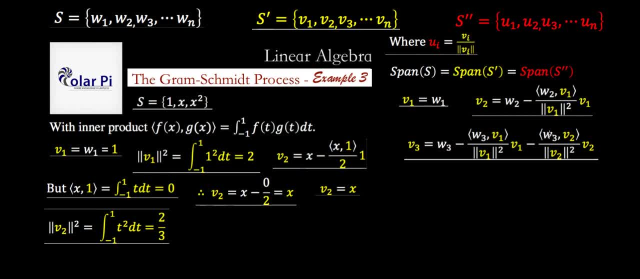 The norm of V2 squared and this inner product and this inner product. Yeah Well, the norm of V2 squared is this here, And that's again because F of X would be V2 and G of X would be V2.. And so 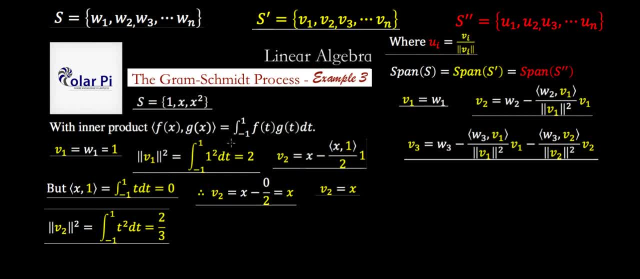 that would be T times T here And that's T squared. And so if you do the integral here, you're going to get two thirds, And it's because it's T cubed over three. Plug in one, you get a third minus. 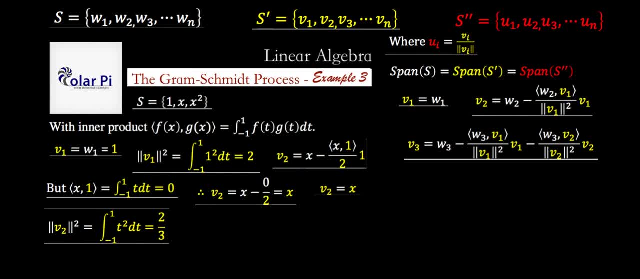 negative: a third, That's a third plus a third, which is two thirds, And so that's going to be two thirds. Right, Okay, cool, cool, All right, And so next we figure out what this is, which is: 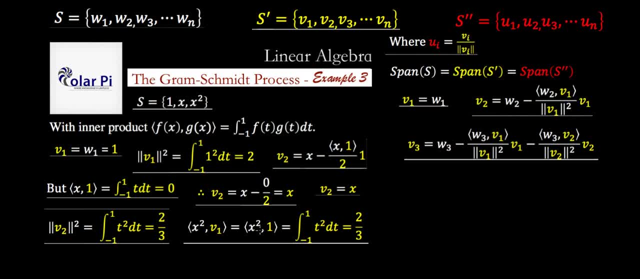 the inner product between W3 and V1.. And so, again, we're using this definition here, But clearly, in here we're going to get T squared times one, And when we integrate we're going to get two thirds. And so, yeah, like- and it just coincidentally turned out to be the same as this here, But yeah. 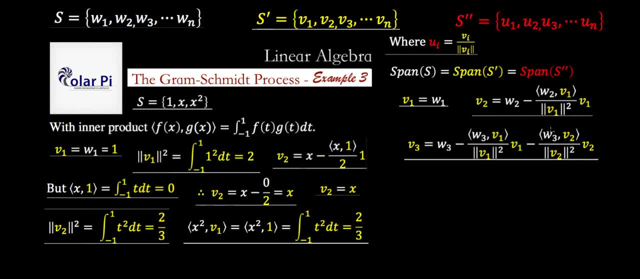 okay, next we're going to need to figure out what this inner product is, right there, right, Okay, cool, And this inner product, right there, is going to be. it's going to be this here, right, And V2 is. 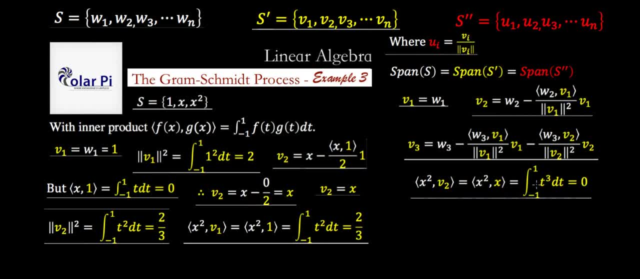 X and W3 is X squared, So we get T squared times T, which is T cubed. Earlier I stated that the integral from negative A to A of any odd function, ie T cubed, is going to be T squared times T. 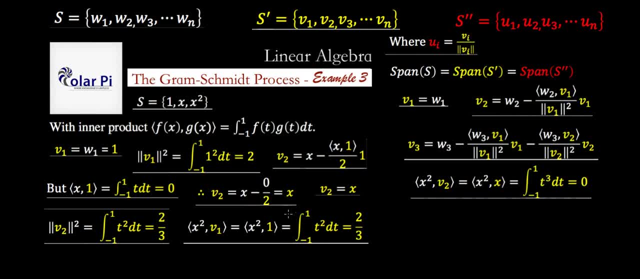 T cubed is equal to zero, So we're going to use that here. Yeah, okay, cool, cool. So now we know all the pieces to figuring out what V3 is, So let's get on with it. V3 is this, First, this, which is: 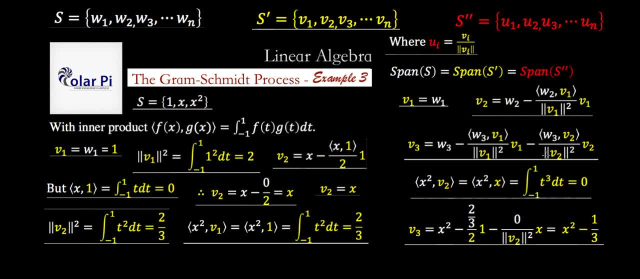 basically substituting in here everything that we've figured out right, And yeah, and once you simplify, you get this for V3. And that's that. So we already had that. V2 is X squared times T squared, And from the start we knew that V1 was one, And we have here what V3 is. So we're done with the Vs.